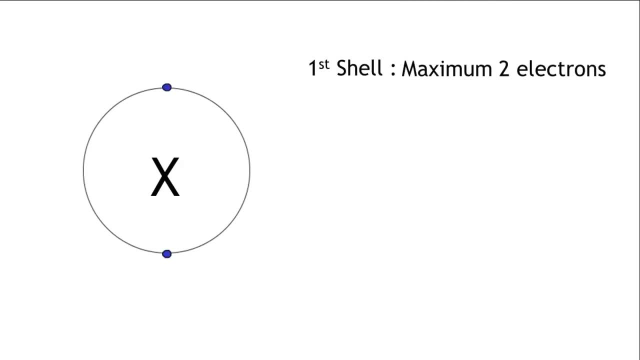 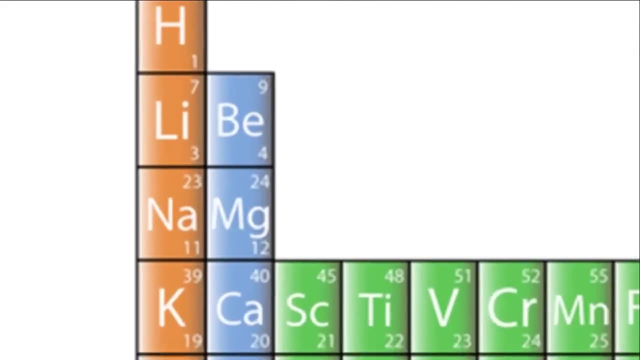 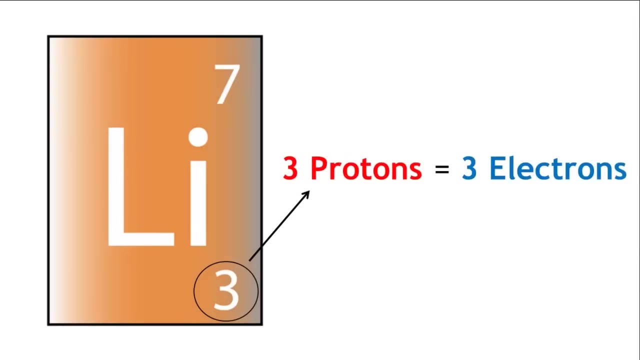 innermost shell can only hold a maximum of two electrons. The shells which come after this can hold a maximum of eight electrons. Let's look at some arrangements. Lithium has three protons, Therefore it has three electrons. The first two electrons are placed in the first shell, closest to the nucleus. 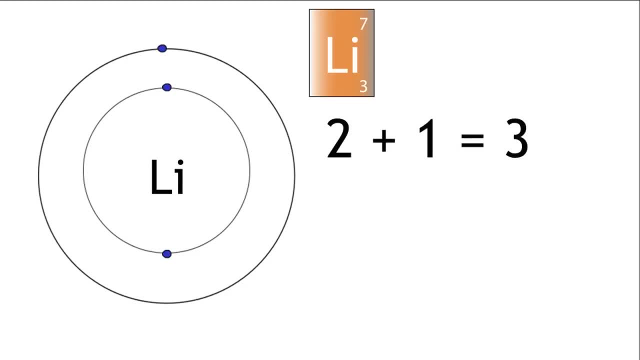 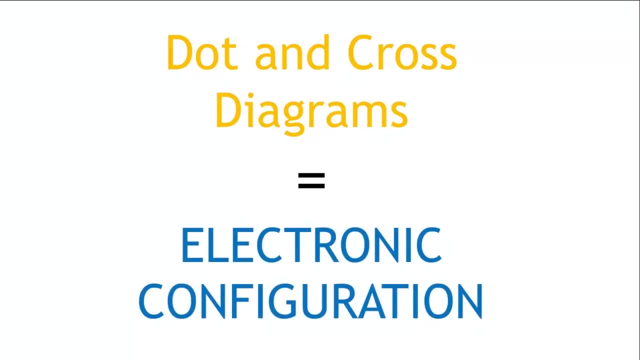 and the third electron is placed in the second shell. Two plus one, three electrons. These diagrams are called dot and cross diagrams, and they are used to show the electronic configuration of an element. You need to be able to draw these diagrams as well as being able to write the electronic configuration in a written form. For lithium, 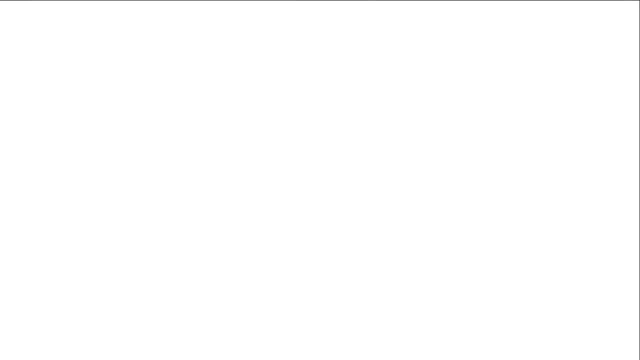 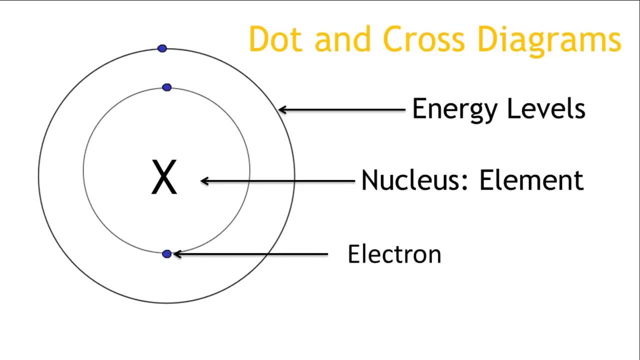 this will be written as Li 2: 1.. In the diagram, the nucleus is represented by the element symbol or a central black dot. The energy levels are represented by circles around the nucleus and the electrons are represented by dots or crosses. 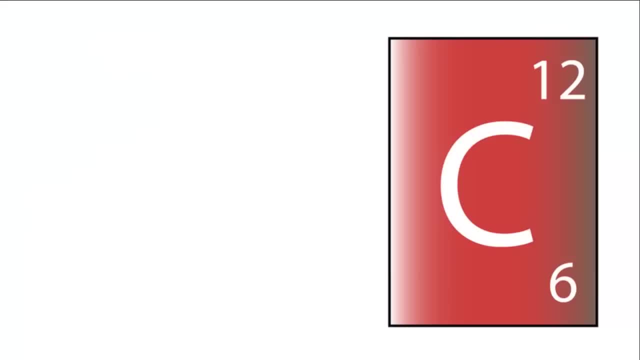 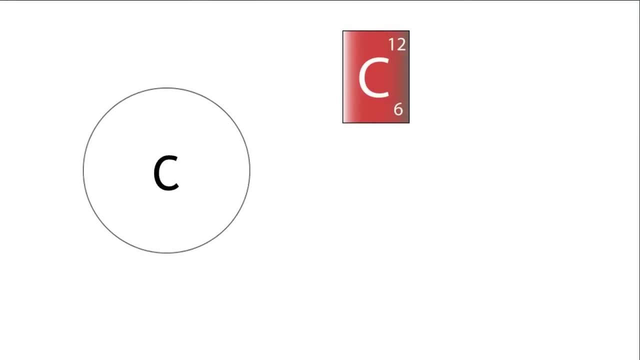 Let's look at some more examples. Carbon has six protons, Therefore it has six electrons. The first two electrons are placed in the first shell and the next four are placed in the second shell. Two plus four, six electrons. This will be written as C 2. 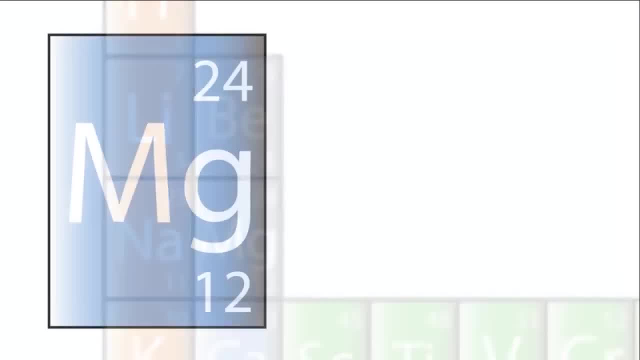 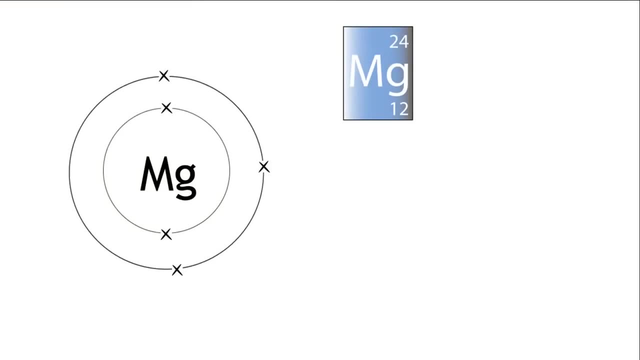 4.. Magnesium has twelve protons. Therefore it has twelve electrons. The first two are placed in the first shell, the next eight are placed in the second shell and the last two are placed in the third shell. Two plus eight plus two Twelve electrons. This will be written as Mg 2 8- 2.. The organisation: 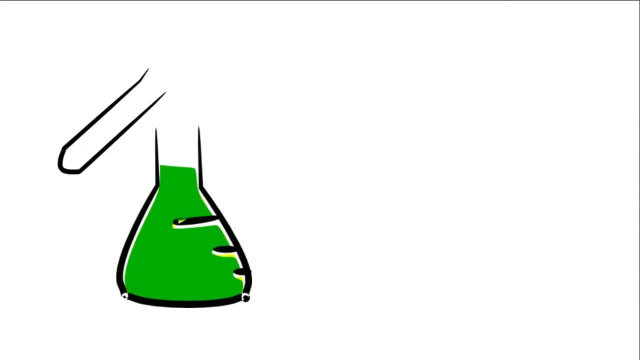 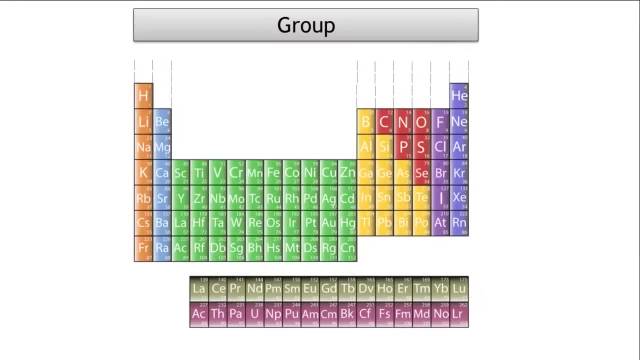 of these energy levels is what gives elements their different reactivities. The number of electrons in the outer shell of an atom tells you the group number to which they belong on the periodic table. Members of the same group with the same number of electrons in. 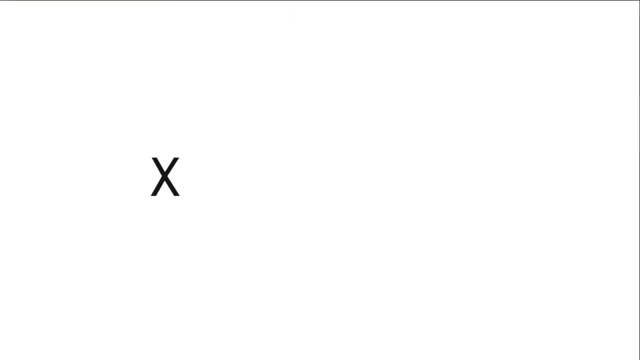 their outer shell have similar reactivities, So electrons are arranged in shells, or energy levels, around the nucleus. Each energy level has a maximum number of electrons it can hold. The lowest energy level is always filled first and can only hold two electrons, while the